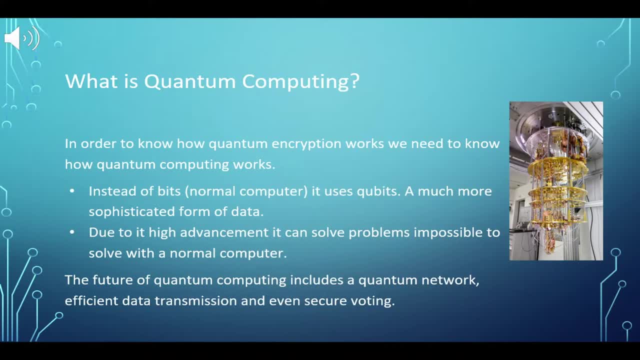 which is a much more sophisticated form of computing. It's a much more sophisticated form of data in order to calculate much higher-level thinking questions and answer a lot of questions that we have, which are impossible to get in today's technology. Qubits work in a way where normal computers' bits use ones and zeros to give us data to read and gives us answers. That's how the computer takes in information and spits it out. 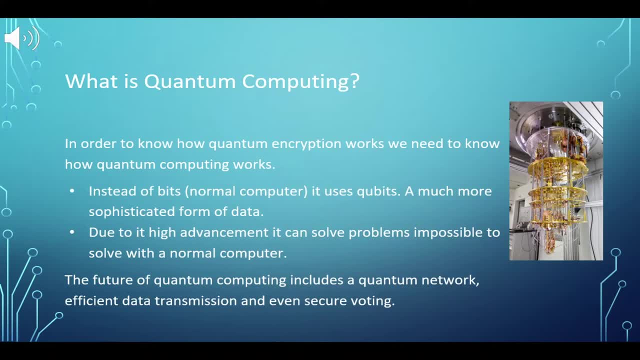 What qubits are? it's the same situation. They use ones and zeros. However, they have the capability to be both at the same time, and when they are both at the same time, a lot of new things can be generated from a computer. 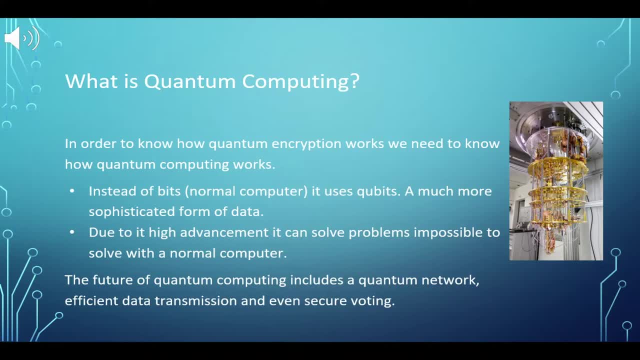 Due to its high advancement, it can solve problems impossible to solve with a normal computer. So, for example, it'd be able to predict the stock market much more accurately than anything we have currently. The future of quantum computing includes a quantum network, efficient data transmission and even secure voting. 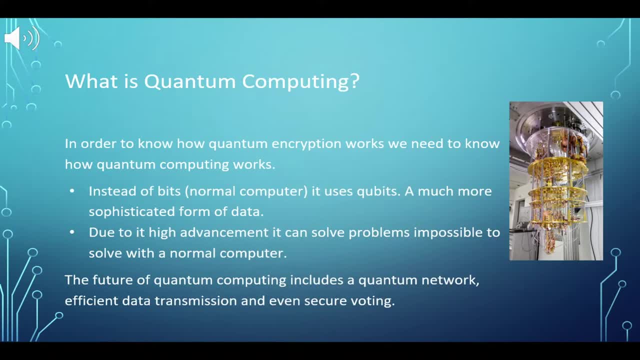 And the neat thing with quantum computing is that it's not just about computing, It's about computing. And the neat thing with quantum computing is that it's not just about computing. It uses quantum physics in order to generate all this new data that we're able to research and develop and come up with new outcomes. 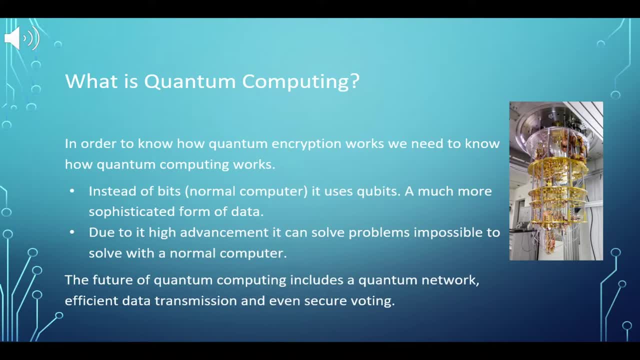 And if you check out our next slide, you'll be able to see a comparison between a normal computer and a quantum computer. When we talk about normal computers, this would be anything such as a smartphone, the laptop that you use or any other technology that we always use. 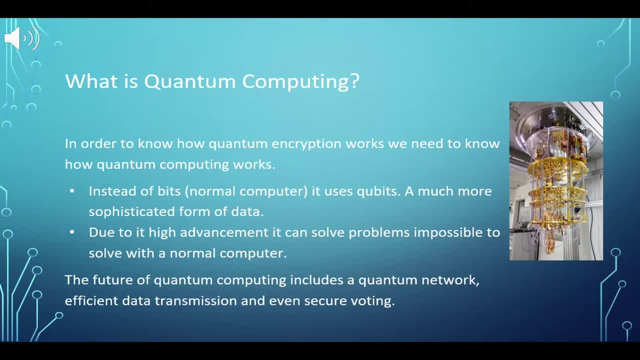 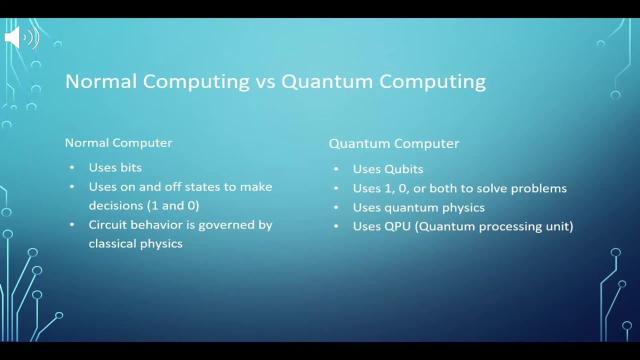 Compared to quantum computing, which I hope in the near future is perfected, so that we can advance our technology in the future. Normal computing versus quantum computing. We've been using computers since the 19th century and right now we're currently on the fourth generation of computers. 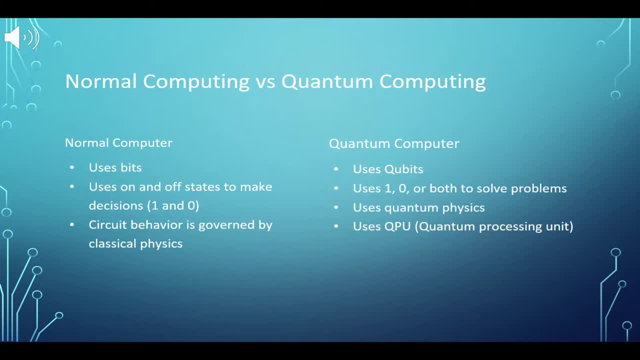 in terms of the microprocessors and transistors and integrated circuits, And currently the fifth generation of computers is being developed, and that's better known as quantum computing. Here we're going to be comparing our current technologies versus the feature computing that is quantum computing. 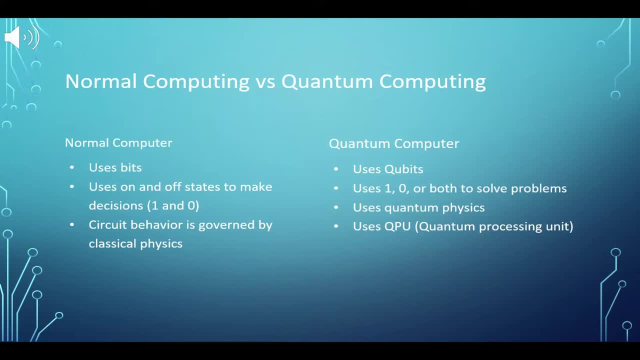 Normal computers use bits, whereas quantum computers use qubits. Bits is where it's an on-off state, where it's either a 1 or a 0, and qubits can be a 1 or a 0 at the same time. 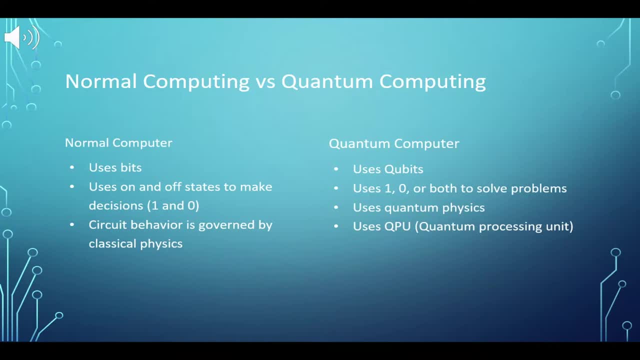 This allows us to solve more complex problems and have a completely different structure for how data can be processed. Conventional computing is based off of classical phenomenons like electrical circuits and just being in on-and-off states, whereas quantum computing uses quantum mechanics such as superpositioning and entanglement. 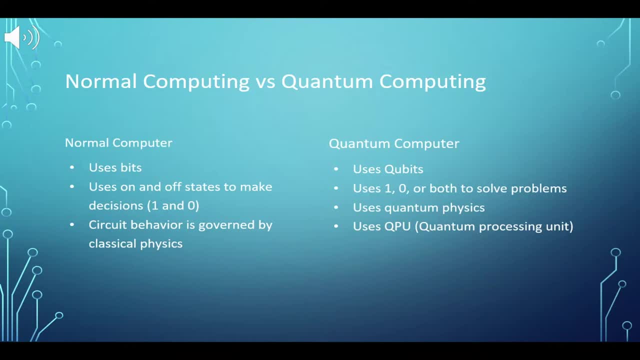 This essentially allows for more than one state to be possible at the same time. Also, in conventional computing, information storage is manipulated. It's stored in bases of bits based on voltages and lower-high charges, where a low charge is 0 and a high charge is 1.. 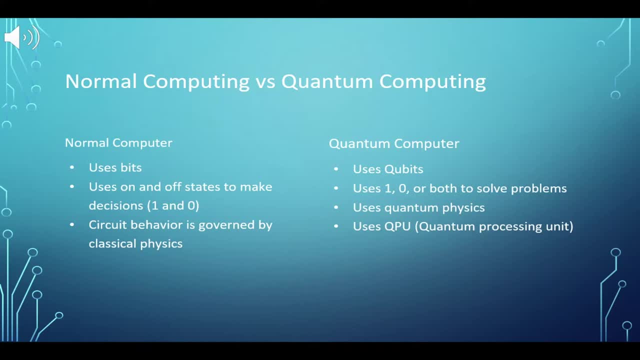 And information storage in quantum computing is stored, as in qubits, which is based on the spin of the electron or the polarization of a single photon. Classical computing also is governed by classical physics, whereas quantum computing is going to be governed by quantum mechanics. 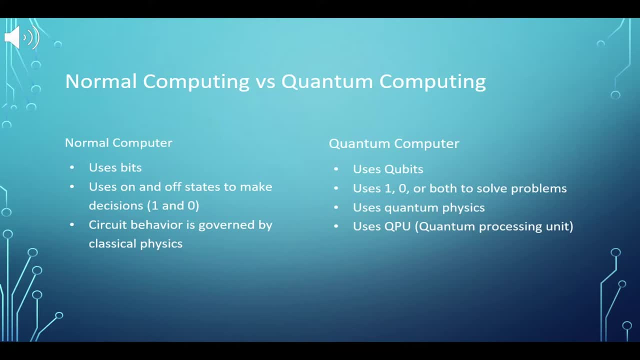 which is based on the spin of the electron or the polarization of a single photon. In quantum computing, data processing is done using a CPU, which is a central processing unit, where it consists of arithmetic logic units and process registers and a control unit. 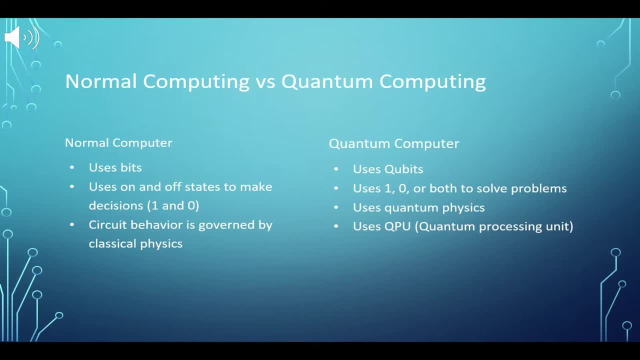 And in quantum computers, data processors are done in the quantum processing unit, or the QPU, which consists of numbers that are interconnected- qubits. In the next slide, you'll see a YouTube video that'll help summarize quantum computing, as it can be a confusing topic. 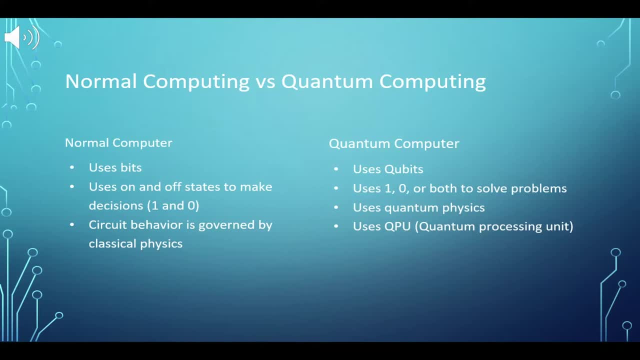 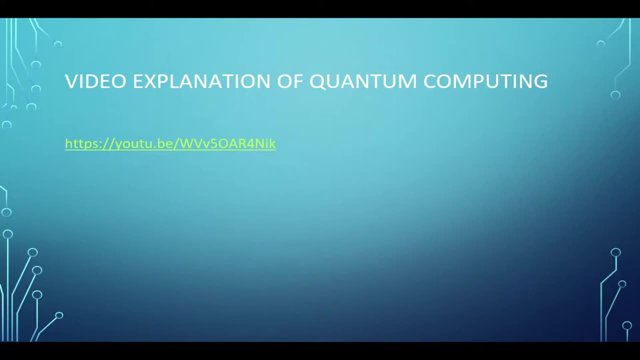 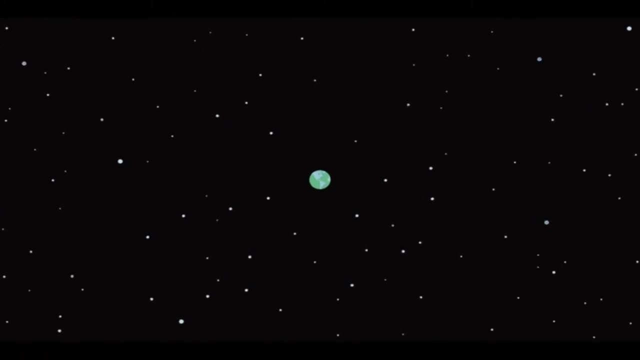 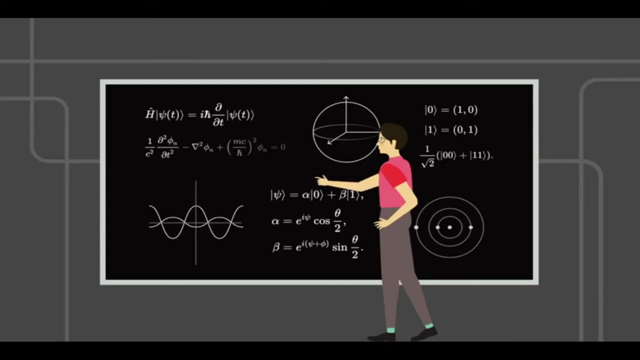 Hopefully, the video will sum up any questions you have and explain it in a more understandable way. Quantum physics, one of the most successful theories of modern science, describes the way our world works at the most fundamental level. Quantum computing has become one of the leading applications. 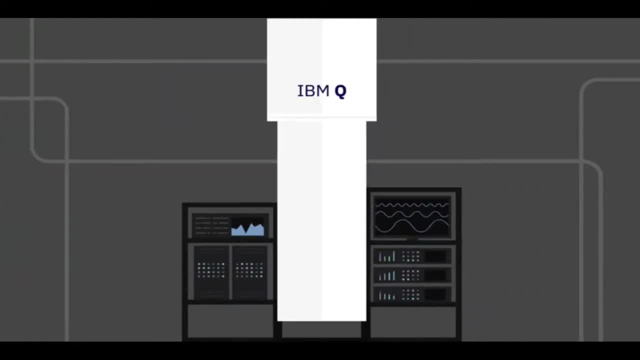 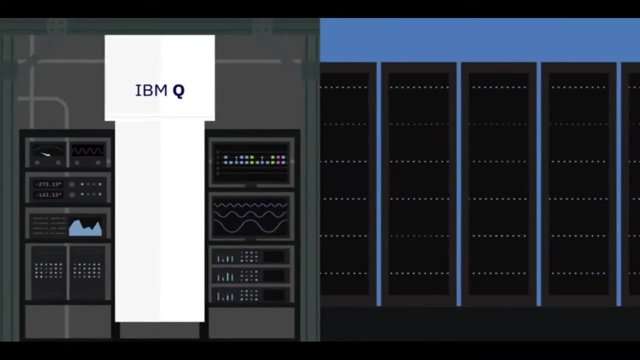 of quantum physics. Quantum computers have the potential to solve some of the world's most complex problems that are beyond the reach of even today's most powerful supercomputers. Quantum computers are not going to replace classical computers, but their radically different way of operating. 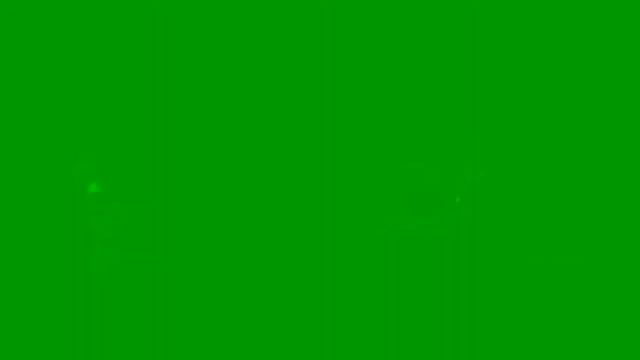 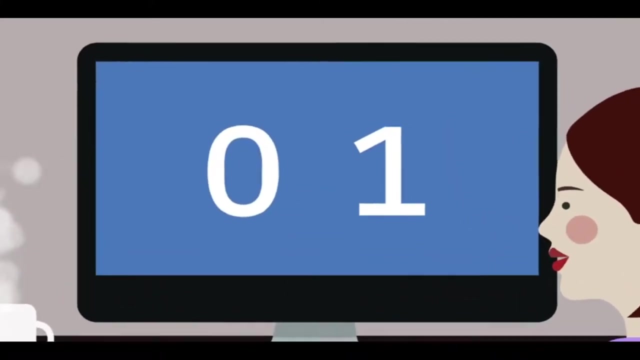 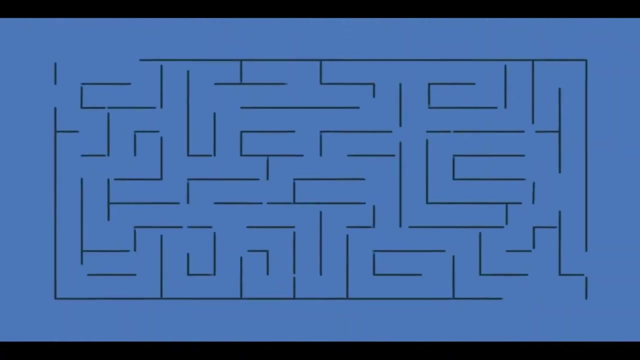 enables them to perform calculations that classical computing cannot. Let's see how they differ. Classical computers encode information in bits, and each bit can represent a zero or a one. These zeros and ones act as on-off switches that ultimately translate into compute functions. 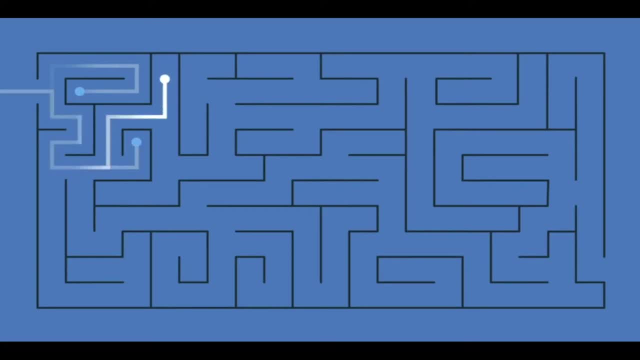 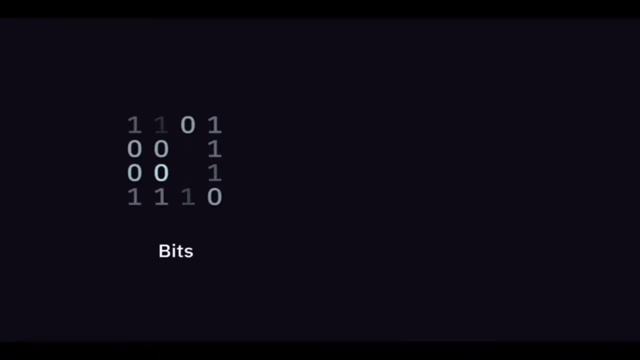 To perform a simple calculation, like solving a maze. a classical computer would test each possible root, one at a time, to find the correct one. Just as classical computers have bits, quantum computers have qubits. Qbits, however, make use of two key principles of quantum physics. 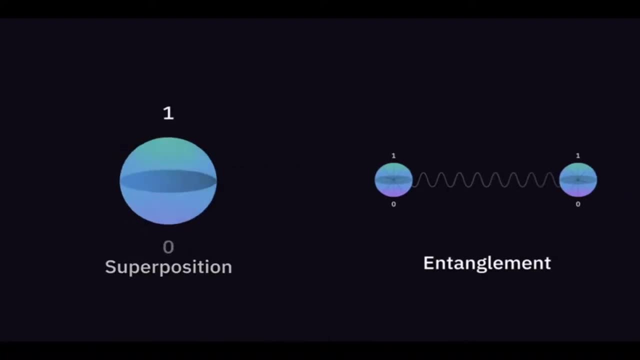 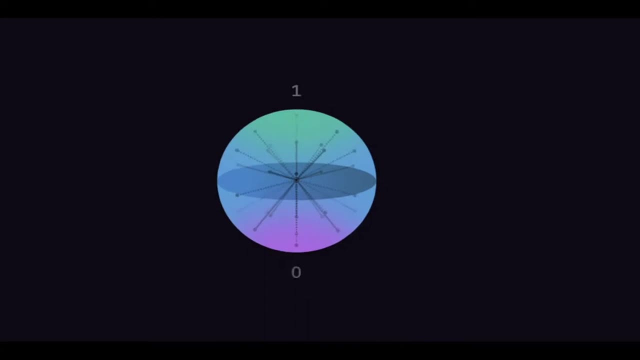 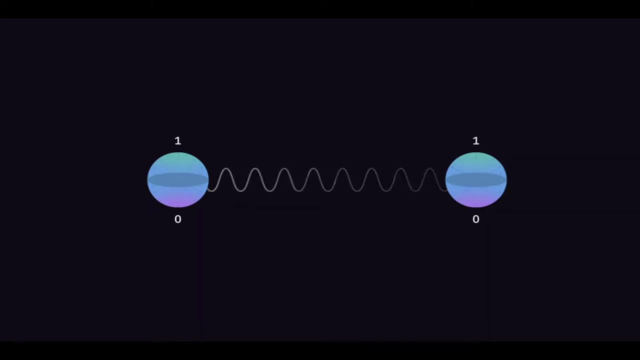 superposition and entanglement. Superposition means that each qubit can represent a zero, a one or both at the same time, And entanglement happens when two qubits in a superposition are correlated with one another, Meaning the state of one, whether it's a zero, a one or both. 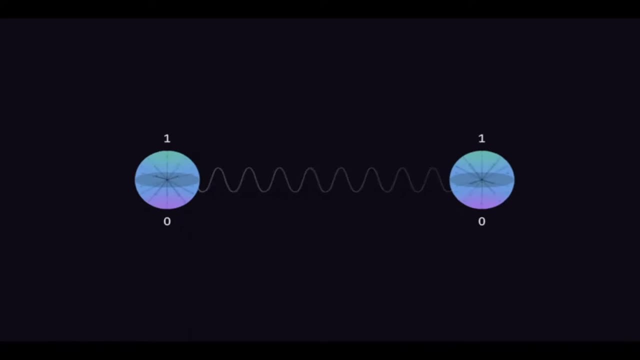 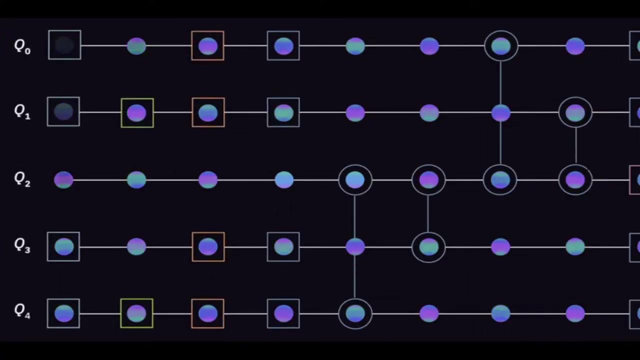 depends on the state of another. Using these two principles, qubits can act as a much more sophisticated version of switches, helping quantum computers solve difficult problems that are virtually impossible using classical computers. To illustrate how this makes quantum computers more powerful, let's look at some numbers. 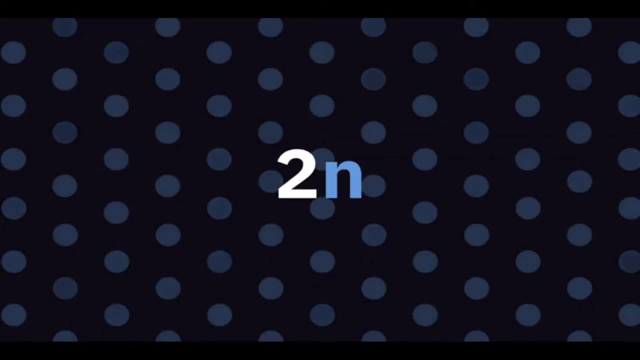 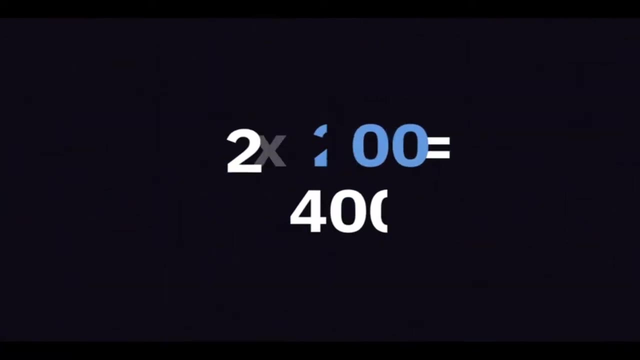 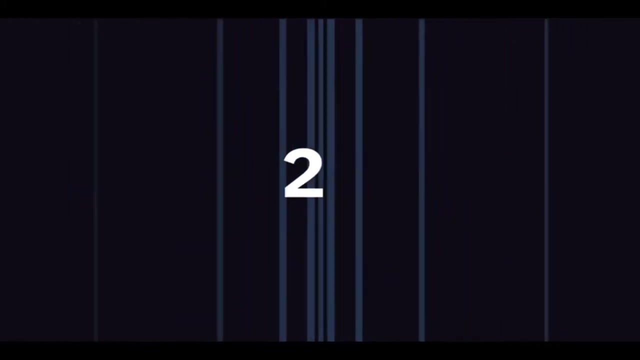 Take a classical n-bit computer, with n representing the number of bits It can represent and examine only one system state at a time. An n-qubit computer, however, would have the power to represent two to the power of n system states and perform parallel operations on all those states at once. 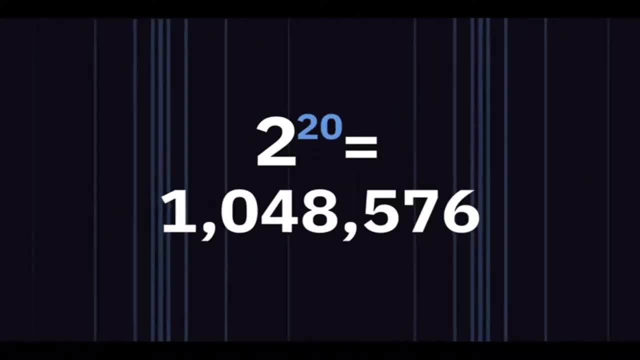 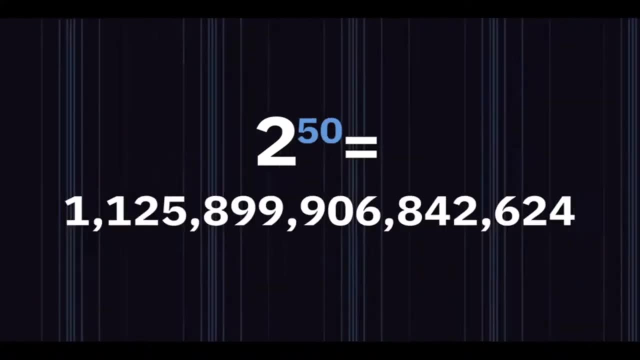 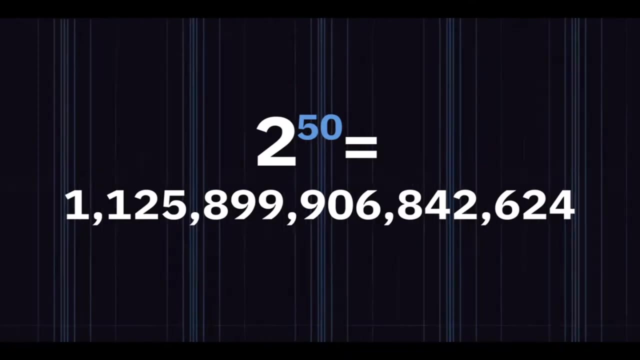 This means that every time you add just one more qubit to a quantum computer, the number of states it can represent and examine doubles. So a 50-qubit quantum machine could examine two to the power of 50 states at once. This exponential increase in power. 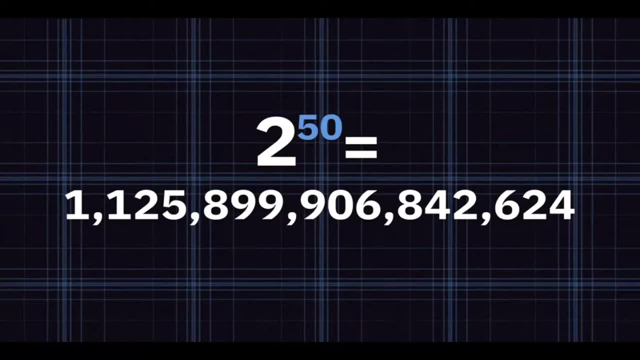 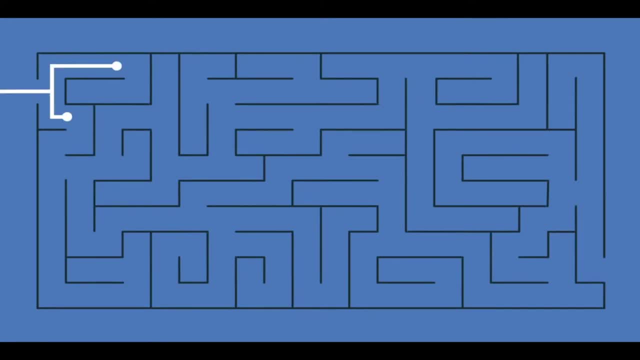 together with the entanglement of qubits, is what allows quantum computers to solve certain problems so much more efficiently. While a classical computer solves a problem like the maze by testing each possible root one at a time, a quantum computer uses its entangled quantum states. 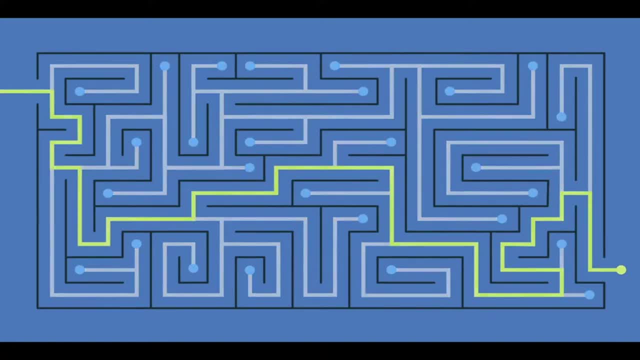 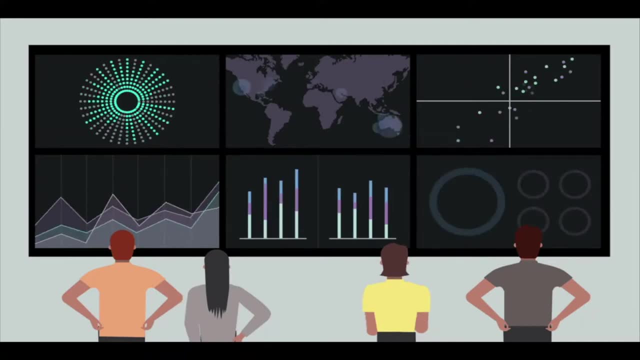 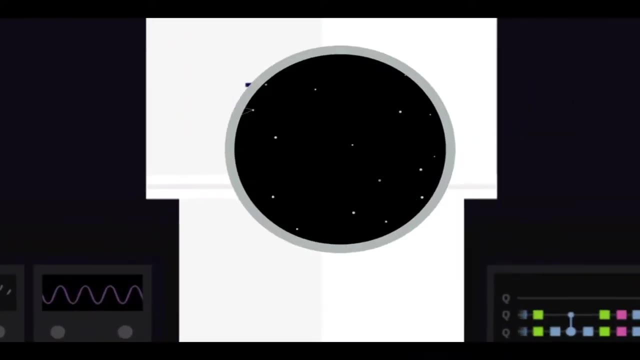 to find the correct root quicker, with far fewer calculations. Think of it this way: Technologies that currently run on classical computers can expertly find patterns and insights buried in vast amounts of existing data, But quantum computers will deliver solutions where patterns cannot be seen because sufficient data does not exist. 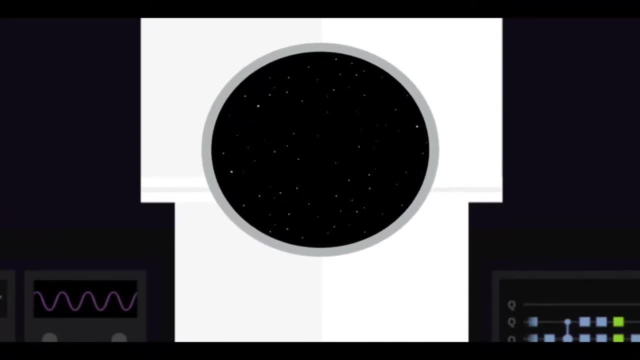 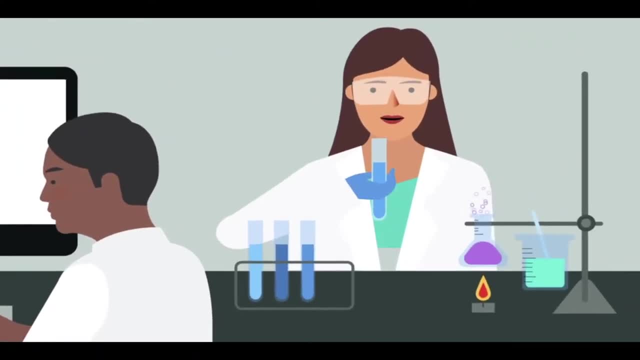 or the possibilities for discovering an optimal answer are too enormous to ever be processed by a classical computer. Quantum computers could lead to the discovery of new medicines and materials by helping us untangle the complexities of molecular and chemical interactions. They could help the financial services industry. 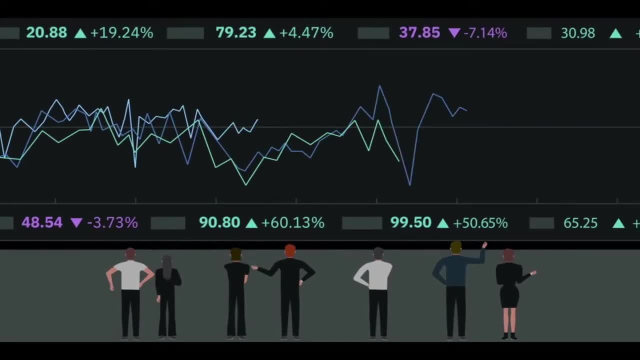 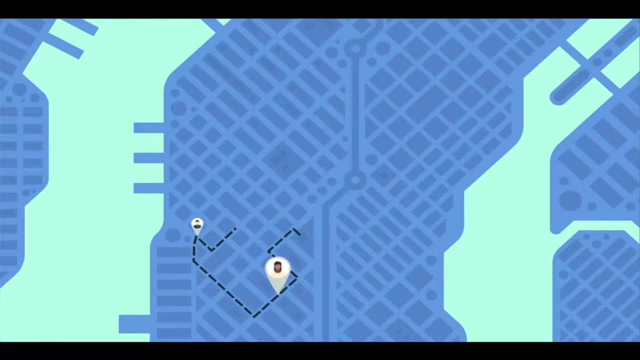 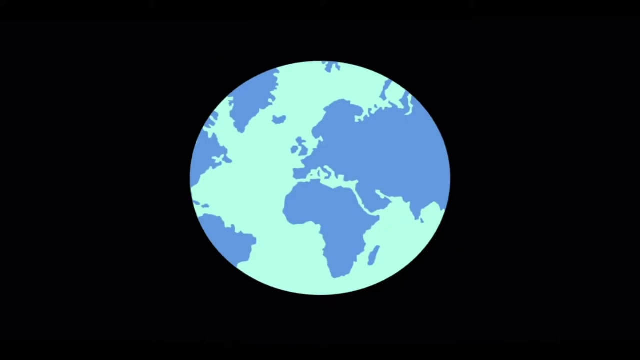 make better investments by finding new ways to model financial data and isolate key global risk factors. They could even transform supply chain and logistics by finding the optimal routes across global systems, like optimizing fleet operations for deliveries during the holiday season. Quantum computing won't replace 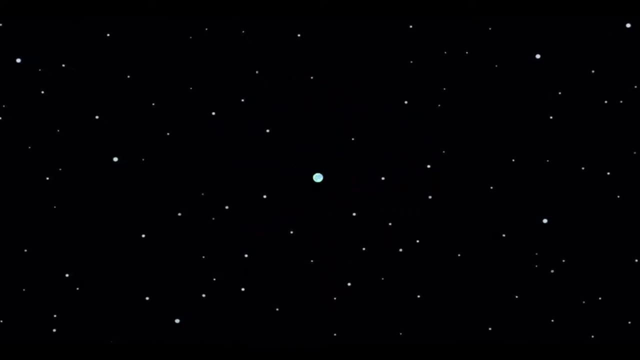 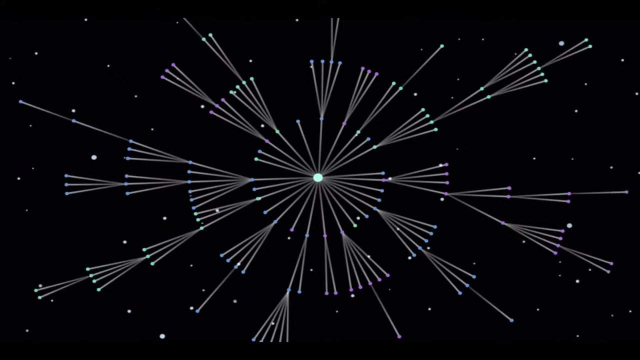 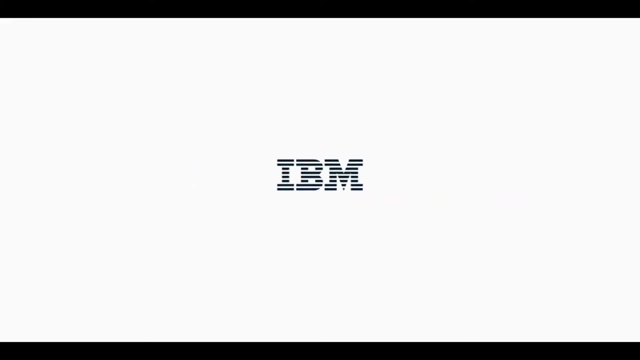 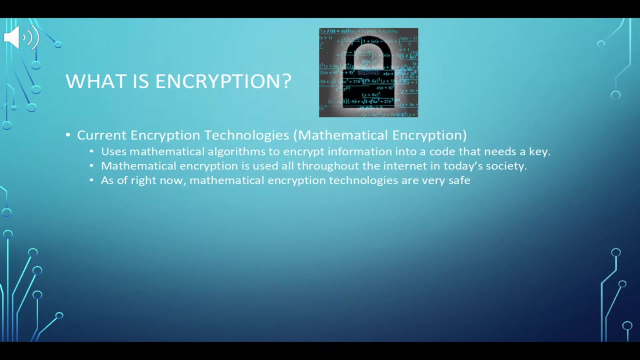 our everyday computers and smartphones, but its ability to solve complex problems will open up a new universe of information, transforming our view of the world and the way we navigate it. So now you know the basics of quantum computing and that's necessary to understand, kind of, where quantum encryption has come from. 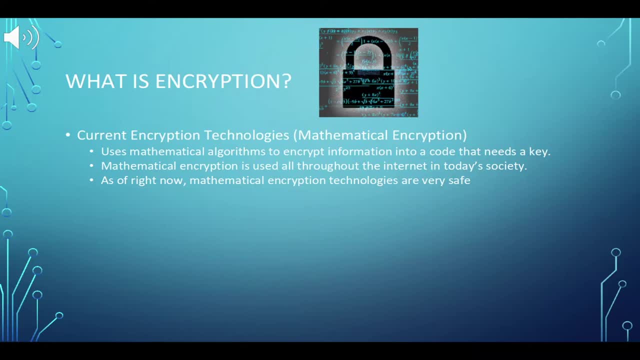 But to first go into that, we need to have a firm understanding of encryption, And I'm sure most of you have a pretty good understanding. but these are mathematical algorithms to encrypt information that use one or more keys. As of right now, these are pretty safe. 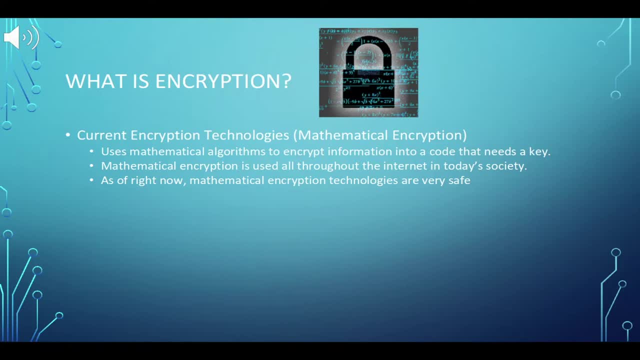 and they are used in everything from email on websites. You've probably heard of algorithms like AES, triple DES- RSA is one of the most popular, as well as elliptic curve cryptography. So far, gradual increases in key links are sufficient to compensate for technology advances. 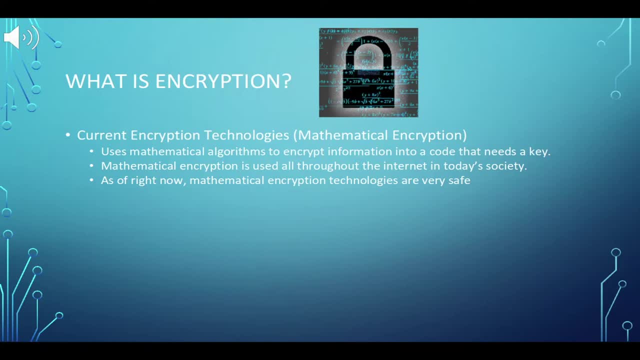 But quantum computing is something that could absolutely break our current encryption algorithms. For example, researchers at Google and the Royal Institute of Technology have developed a quantum system that could crack a 2,048-bit RSA in a roundabout way, And it can be done in about 8 hours. 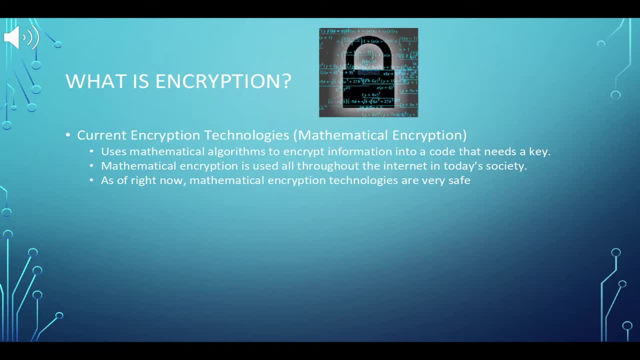 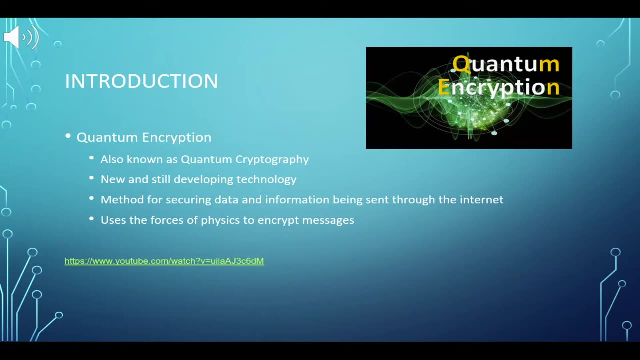 So that kind of gives you a picture of where technology is headed and where encryption is headed. So now that we know how normal encryption works with our standardized computers that we use on a day-to-day basis, let's talk about how it competes with quantum computers and for them. 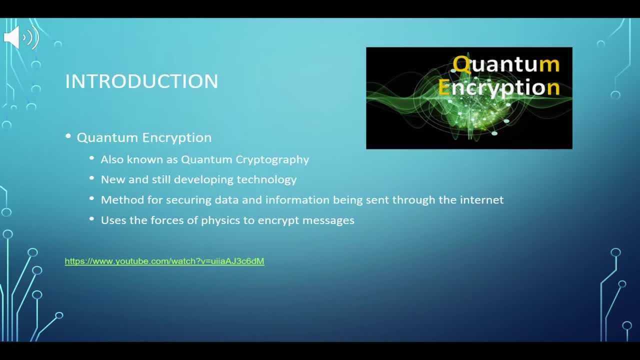 So it's also known as quantum cryptography. It's new and still developing throughout the world. There's multiple continents looking at this all over the world. It's a method for securing data and information being sent through the internet, and it uses the forces of physics. 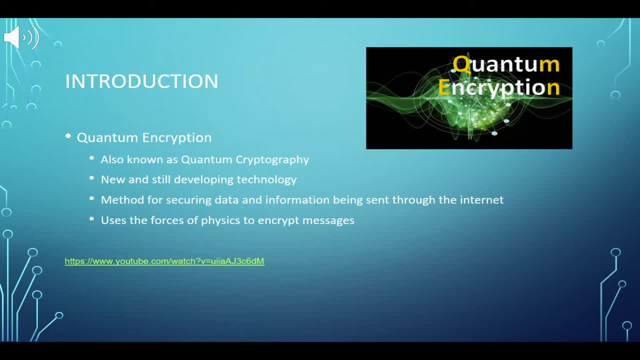 to encrypt a message. The importance of quantum computing is to make sure that anything that you're sending that needs to be encrypted obviously cannot be read from anyone that it's not intended to. So with quantum computers, it's very easy to decrypt a message. 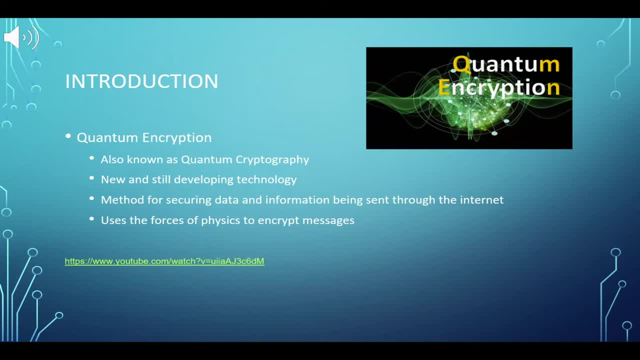 That's why quantum encryption is important and that we should prepare for it for the near future, so that we can stay safe on the internet and always protect our data. In this slide, you'll see a hyperlink to a YouTube video. The YouTube video talks about quantum encryption. 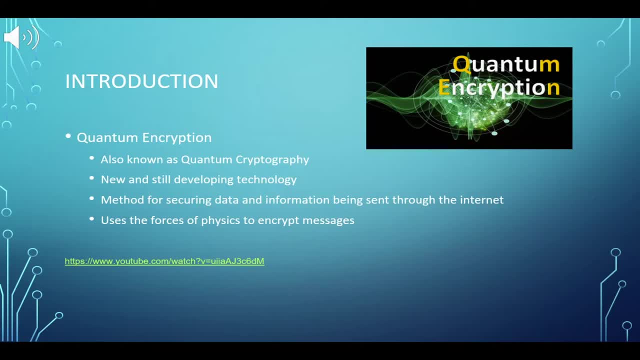 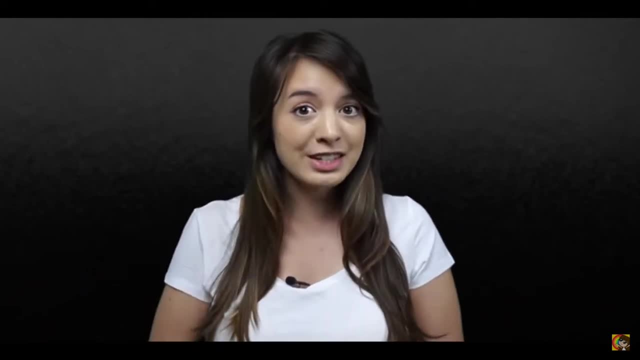 from a different perspective and hopefully it's more easier to understand. It's called quantum cryptography, and what makes it so powerful is that, instead of math, it relies on the laws of physics, One law in particular: the Heisenberg uncertainty principle. 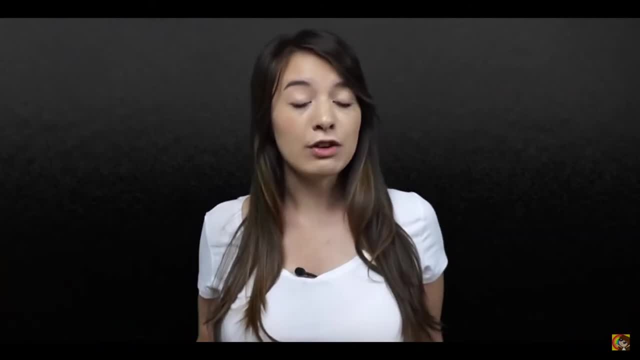 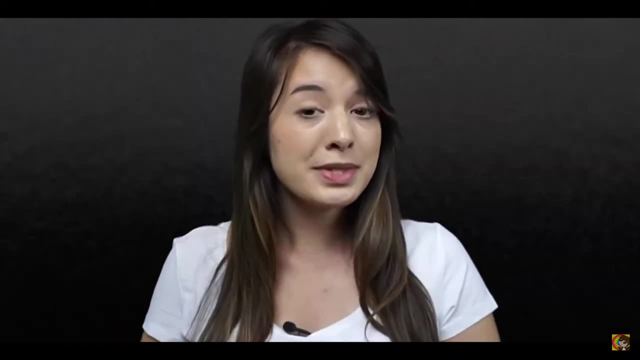 It says that you can't know absolutely everything about the state of a quantum particle. It's not because you're not smart enough or your equipment isn't good enough. It's just because nature keeps some things hidden. Take this scenario: You want to send Bob a private message. 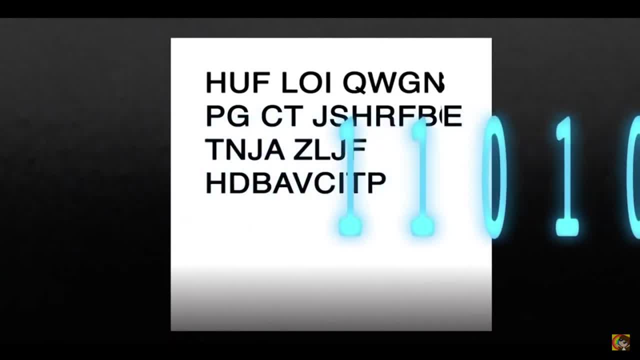 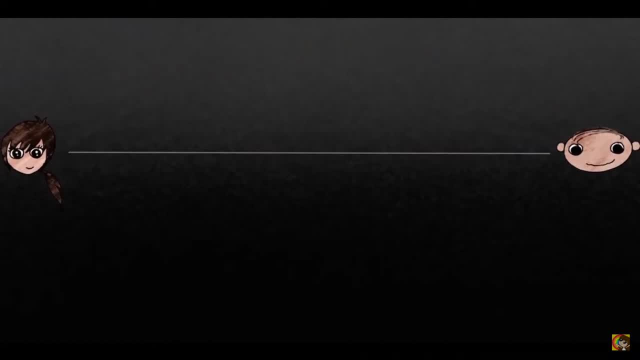 You encrypt the message using a key made up of ones and zeros. You send the key to Bob by a secure line- this could be email or wire- and then mail the message to Bob. Remember, it doesn't matter if anyone else reads the message. 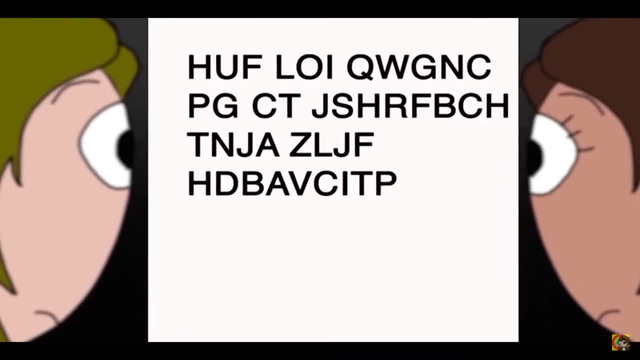 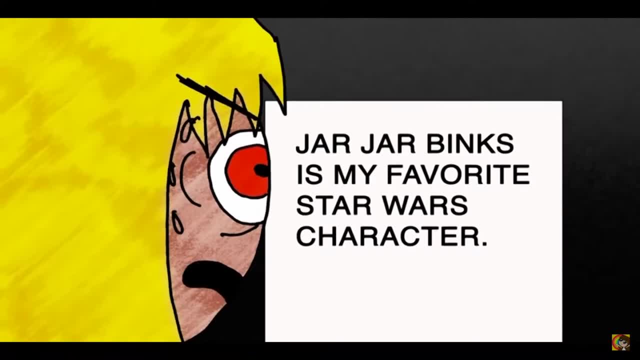 They won't be able to understand it. What's important is that no one sees the key, But an eavesdropper. Eve has tapped into the secure line. Once she has the key, she can read the message and your secret will be publicly known. 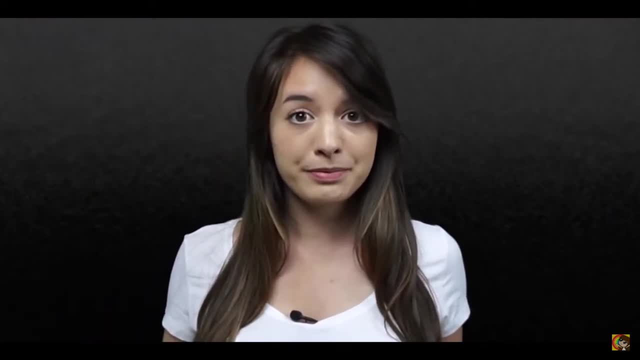 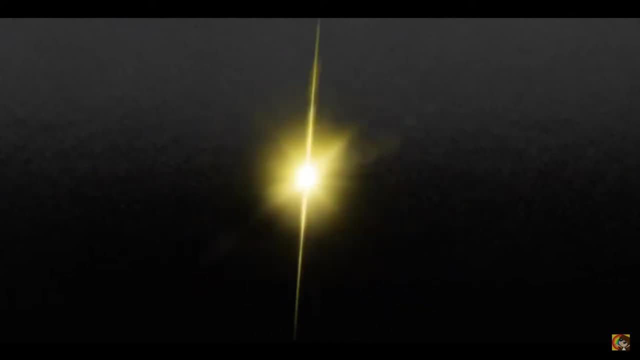 This would never happen if you'd used quantum cryptography. With quantum cryptography, the key is a stream of photons, or light particles. Photons have a property called spin, which can be changed when it passes through a filter. You have four filters: vertical, horizontal and two diagonal. 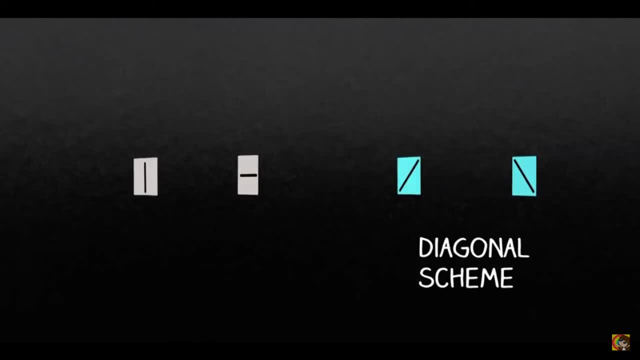 We'll lump these into two groups, the diagonal scheme and the rectilinear scheme, To translate photon spin into a key: a photon with vertical, or this diagonal spin means one and horizontal or this diagonal spin means zero. If you wanted to send 1100,, 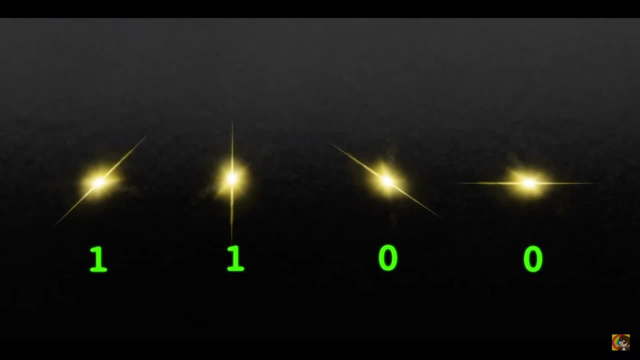 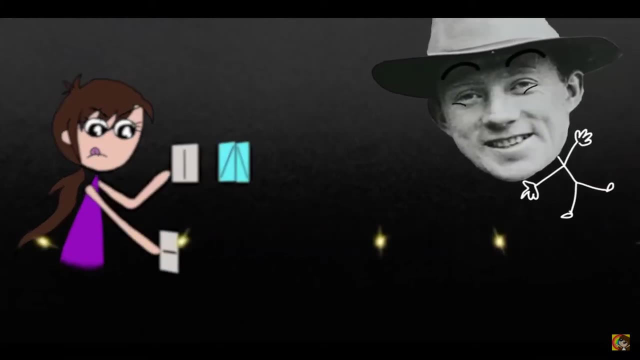 you could send this sequence or this one. You start sending Bob photons switching between filters at random. Now here's where the Heisenberg uncertainty principle becomes important. The only way Eve can measure a photon's spin is by passing it through a filter. 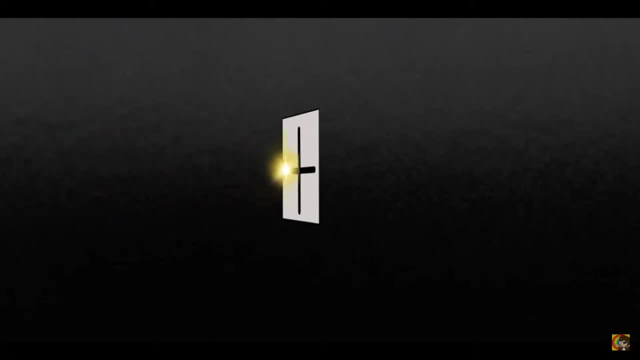 If Eve measures this photon with a rectilinear filter, she'll guess correctly that it has vertical spin and no down a one. But if she uses the diagonal filter, the photon spin will be altered as it passes through. She now incorrectly reads a zero. 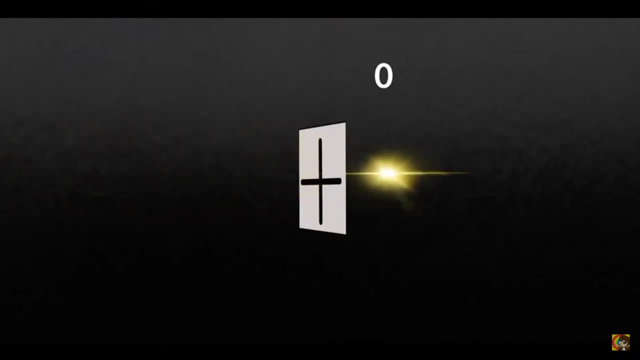 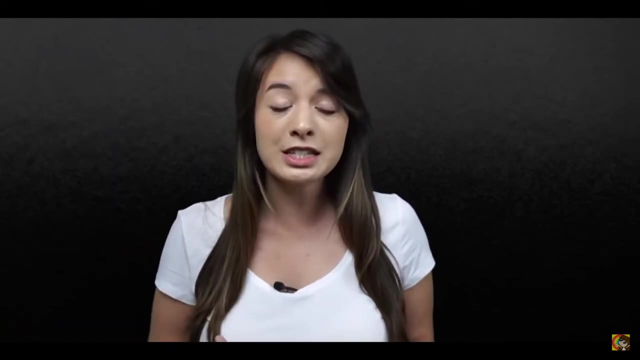 The same will happen if she measures a diagonal photon with the rectilinear filter. Unless Eve knows beforehand which filter to use, she runs a pretty big risk of changing the spin And because you're switching between filters at random, she'll get it wrong about half the time. 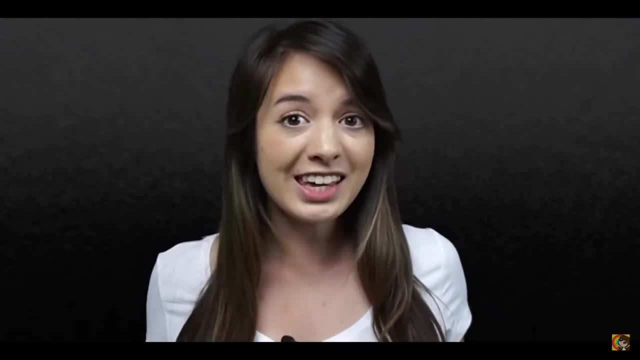 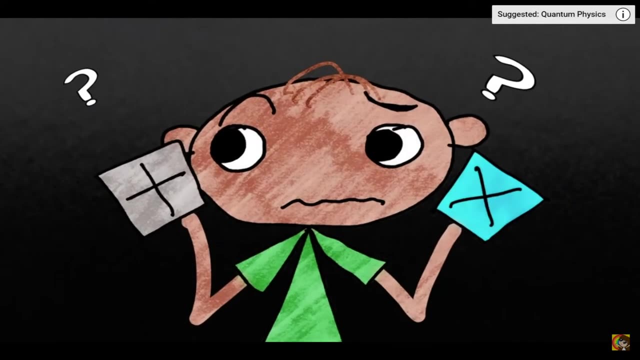 The laws of quantum physics prevent her from knowing the key. Now you may have spotted a pretty big problem. Bob is in the same boat as Eve. He doesn't know which filter to use either. This problem actually took a long time to solve. 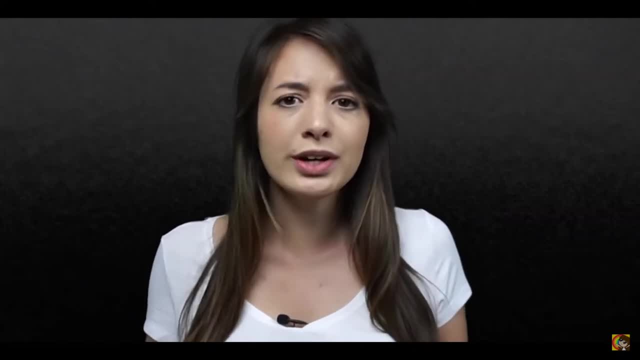 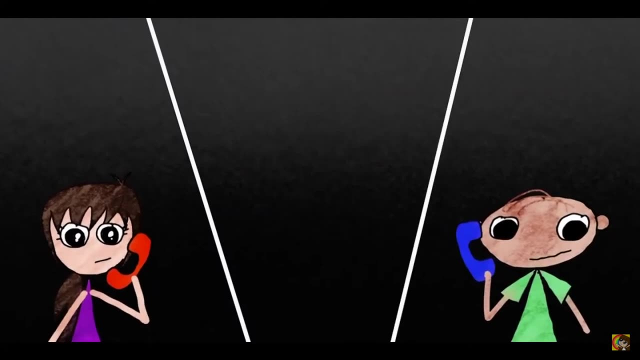 After all, what's the point of a message so secure, even though a saver can't read it? But there is a way around it. After you've sent the key, you call Bob and tell him which scheme you used for what photon. You don't tell him the spin of the photon. 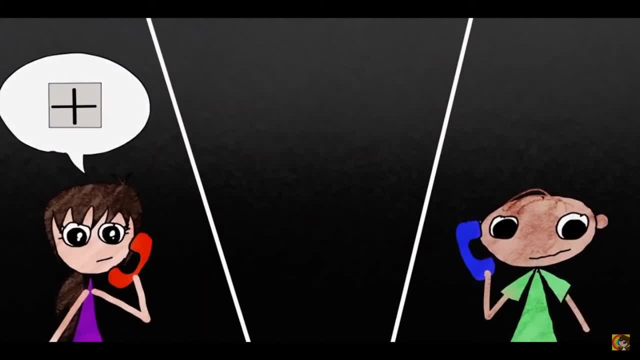 or whether it was a one or a zero, Just whether it was rectilinear or diagonal. If he used the right filter, you both keep the digit. If he chose the wrong filter, you get rid of it. Probability tells us that he got about half wrong. 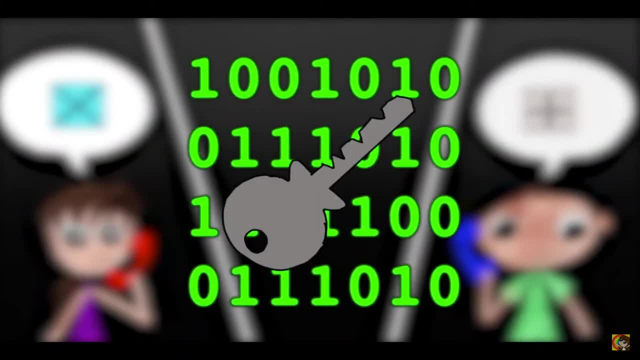 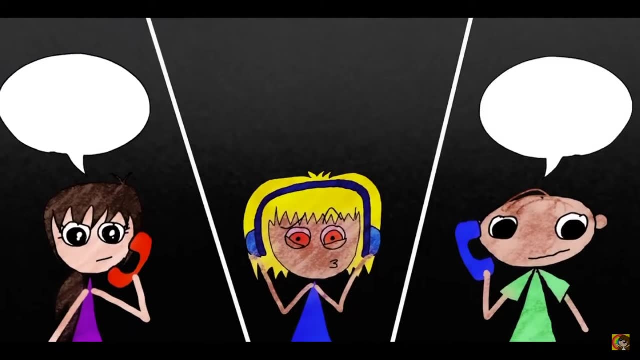 so you keep the half he got right and that's your key. If Eve is listening in on your conversation, it won't help her Say: for the first photon you both used a rectilinear filter, so you keep the digit. Eve used the wrong filter. 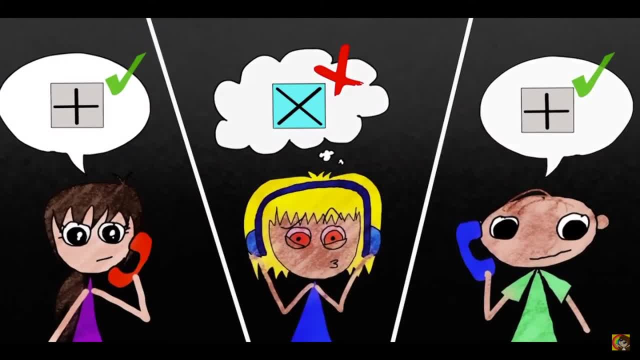 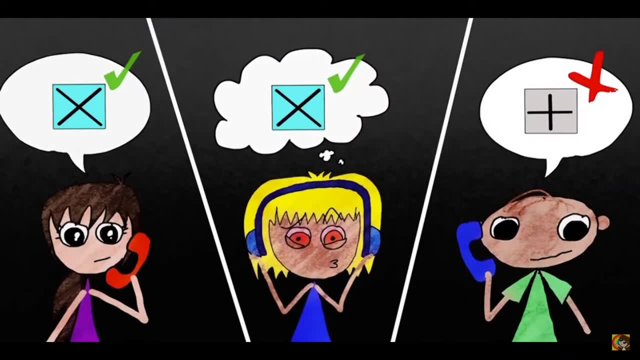 and she can't tell if it's a one or zero from just which scheme you used For the second photon. you used a diagonal filter, So did Eve, But Bob used the rectilinear filter. So you get rid of this answer. So now you and Bob have a totally secure key. 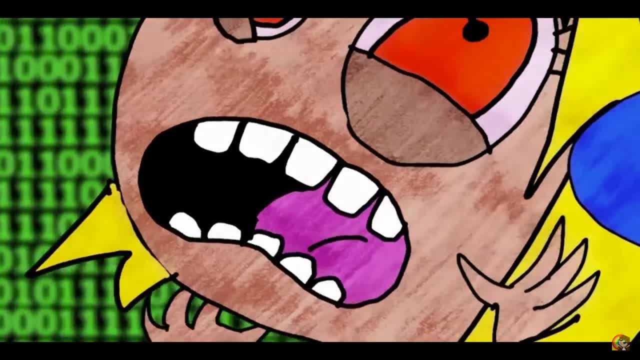 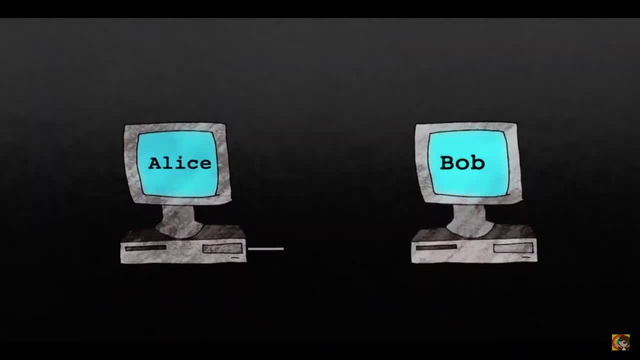 and Eve has a bunch of useless ones and zeros. When the first quantum cryptographic system was tried in 1989, a key was sent 36 centimeters from a computer called Alice to a computer called Bob. Now, newer models have reached 150 kilometers. 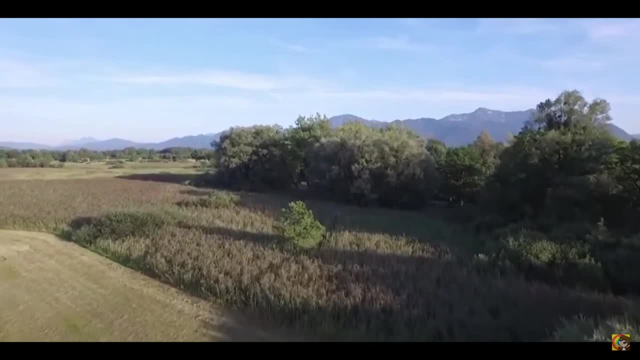 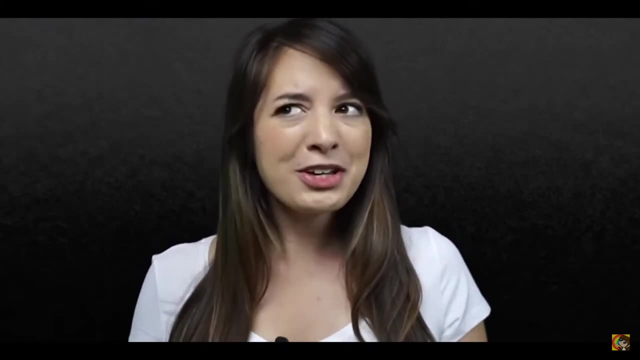 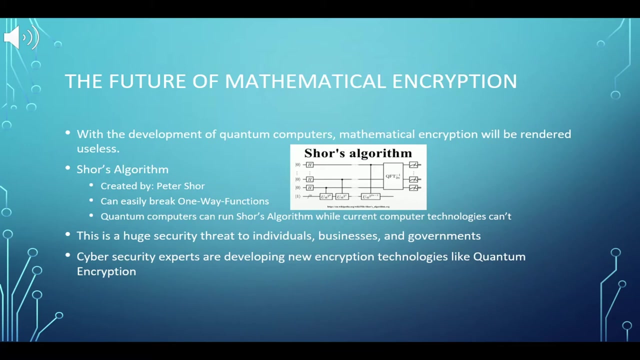 There's still a long way to go, and some people think this is a whole new era for privacy. Quantum cryptography is different from any encryption system before it, So I'm curious as to how the code breakers go about breaking this one. The future of mathematical encryption. 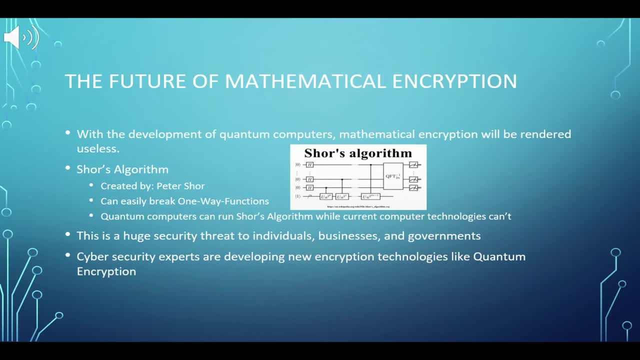 With the development of quantum computing, cracking the mathematical encryption process- those we are currently using right now- could be done within a few minutes. The reason quantum computers can break down mathematical encryptions is due to Shor's algorithm, an algorithm created by Peter Shor. 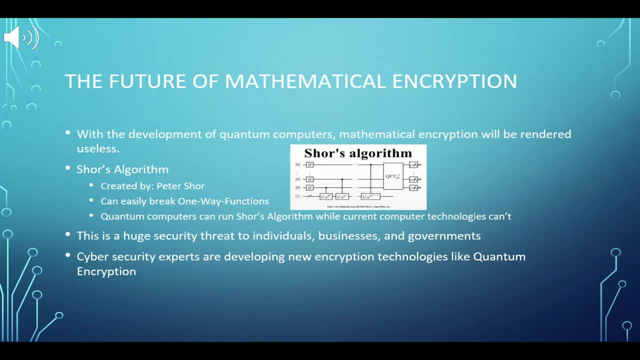 that can break down one-way functions easily. Shor's algorithm can't be run on today's computers, but could easily be run on a quantum computer in the future. This is a huge security threat to all of us, not just on a personal level or for businesses. 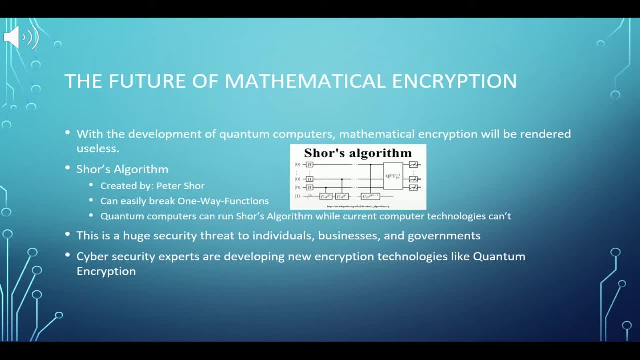 but risking security of the government databases and classified info, as well as military plans and data. Luckily, cybersecurity experts are anticipating this problem and are currently developing new encryption processes that function very differently from our current methods. This new encryption process is called quantum encryption. 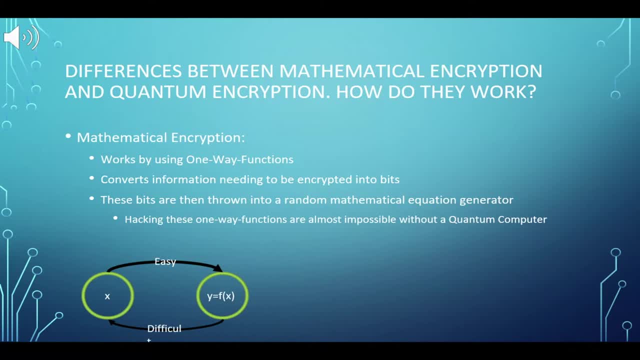 Differences between mathematical encryption and quantum encryption. How do they work? So mathematical encryption works by using one-way functions, also called trapdoor functions. It converts information needed to be encrypted into bits, and then they are thrown into what's called a random mathematical equation generator. 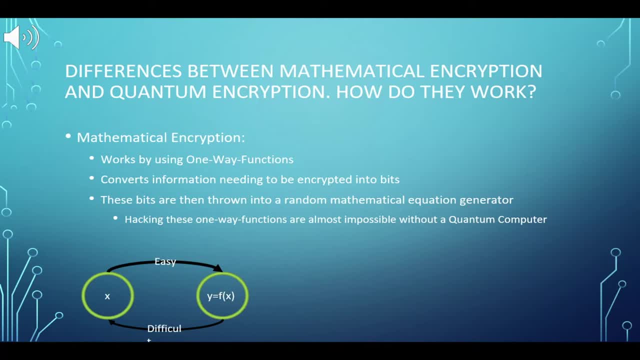 and what we just mean by that is algorithm. Let me give you an example of one of those one-way algorithms, a popular method called RSA. It uses what's called prime number factorization. So, for example, it's easy to multiply two prime numbers together. 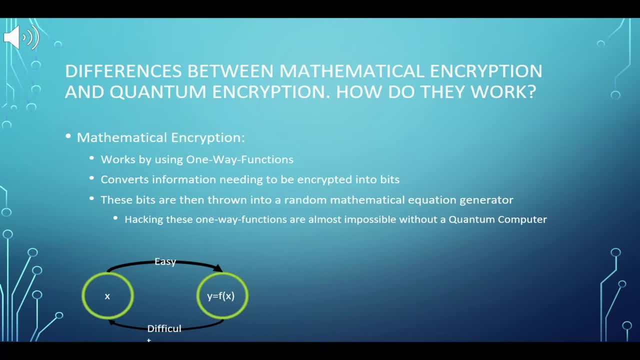 593 and 829, which equals 491,597.. But it's very hard to start with the number 491,597 and work out which two prime numbers must be multiplied to produce it. So using a normal computer to break RSA would take around 300 trillion years. 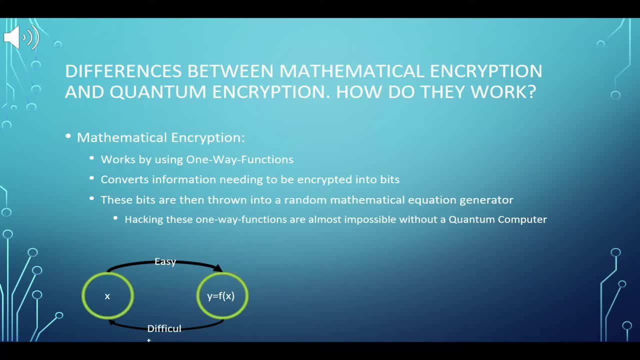 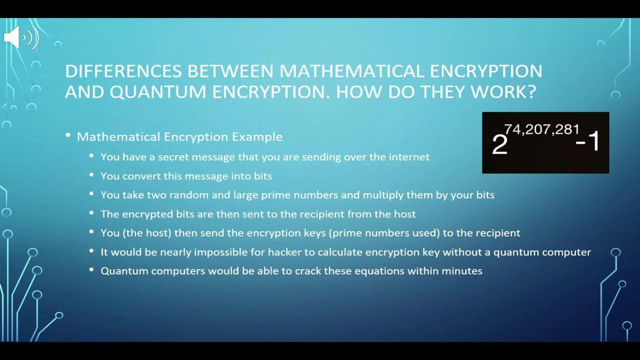 for a regular computer, And that's to specifically break the RSA 2048, which is the current standard. So that's what we mean by saying breaking these one-way functions are almost impossible without a quantum computer. Differences between mathematical encryption and quantum encryption and how they work. 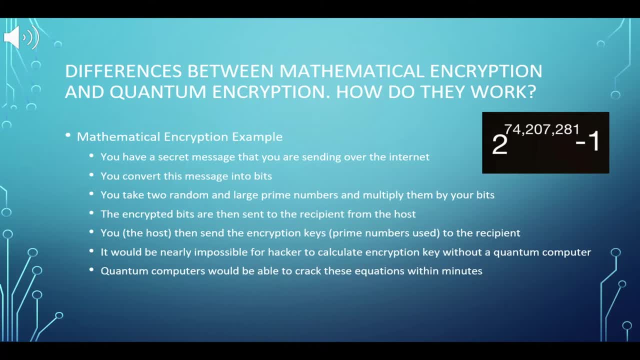 I wanted to cover the first portion, which were the mathematical encryption, which is what we're used to as normal students and computer users. So if I had a secret message that I was sending over the internet and I wanted to say, send it to the professor. 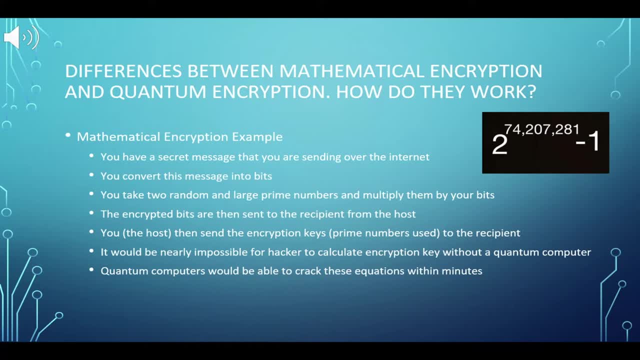 I would have to convert the message into bits. So to do that, you take two random and large prime numbers and multiply them by your bits. The encrypted bits are sent to the recipient or the host, which would be to the recipient from the host. 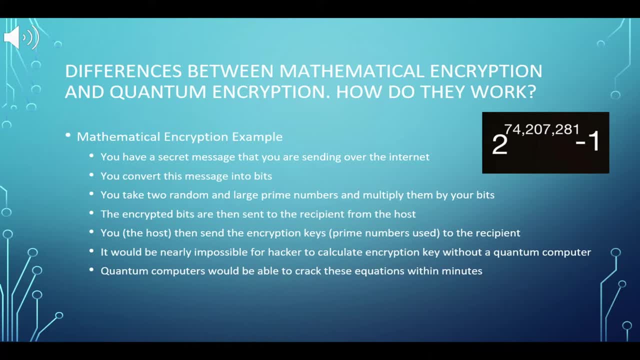 So recipient would be the host, So recipient would be the professor, Host would be me, So me as the host then send the encryption keys, which would be the prime numbers we picked, to the recipient. So I would send the professor something secret. 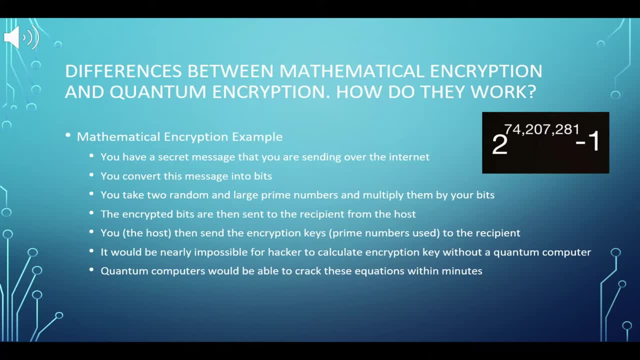 and then I would also give him the answers. to decrypt the message. Now it's important that only he receives the numbers and which would be the key. So, pretty much, if you have a key, you can then unlock a door, For example. 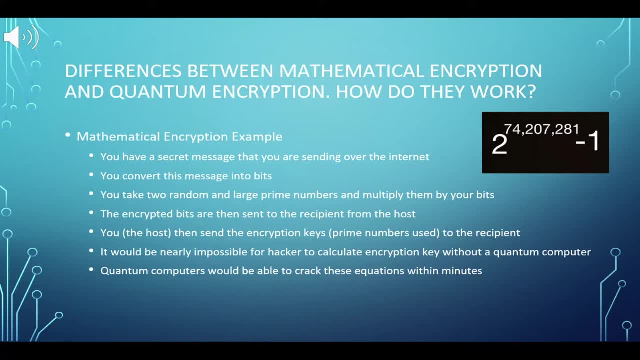 if the professor had the key, he would then be able to unlock the message. So with this type of encryption it would be nearly impossible for a hacker to steal the key or guess the key to get into the computer. With quantum computers it would be extremely easy for it to guess those numbers. 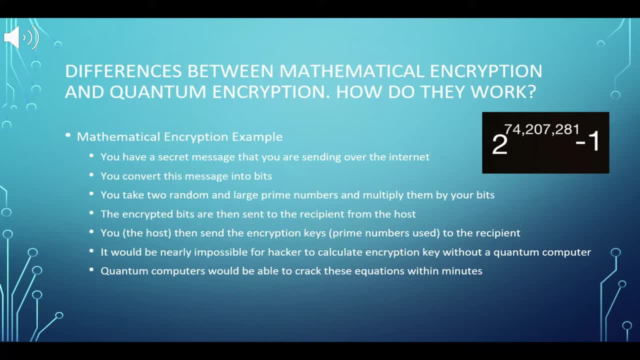 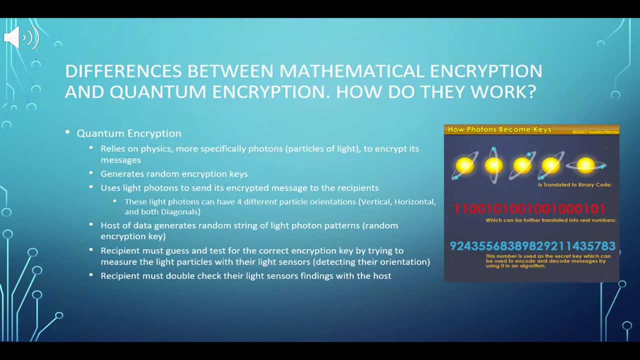 That's how smart a quantum computer is. So the point of this presentation was to bring awareness for quantum encryption, which will be covered on the next slide, and how quantum encryption could then compete with a quantum computer to keep your data safe. This is where quantum encryption comes in. 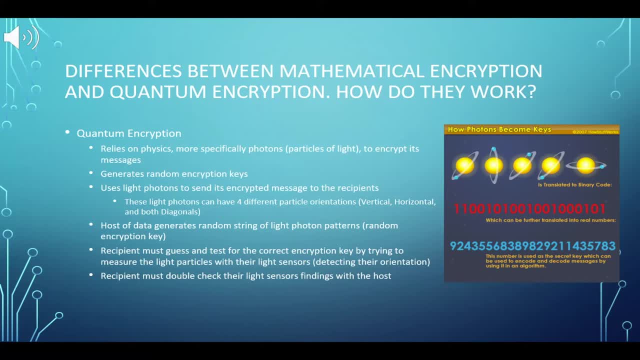 Quantum encryption relies on physics- more specifically, photons, particles of light- to encrypt its messages. rather than using mathematics, Quantum encryption will generate a random encryption key, similarly to how mathematical encryption generates one, but the process of how the recipient gets the key is different. 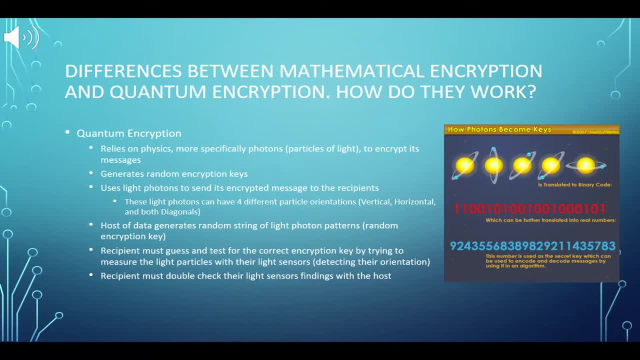 Quantum encryption uses light photons to send its messages. These light photons can have four different orientations: vertical, horizontal and both diagonals. The host of the encrypted data will generate a random string of light photon patterns, random encryption key, and the recipient must guess and test for the key. 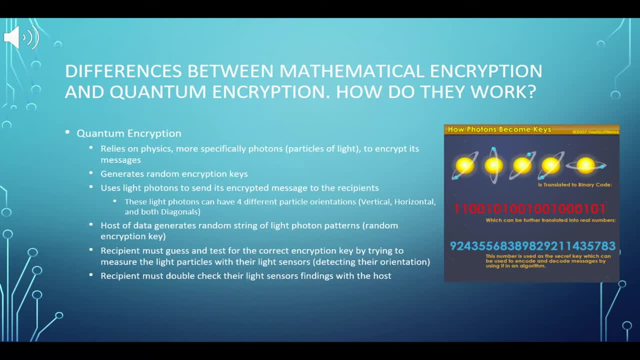 while the host lets them know if they're right or wrong. These light photons run through the recipient's light sensor to try to detect their orientation. There are two different types of light sensors: one that is able to detect the vertical and horizontal orientations of the light photons. 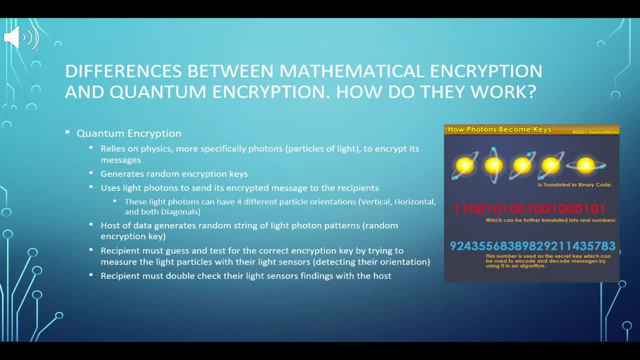 and one that is able to detect the diagonal slopes of the light photons. When the light photon passes through the light sensor, it either passes through with no problem, signaling to the recipient its correct orientation, or it passes through the light sensor and changes its orientation without the recipient knowing anything went wrong. 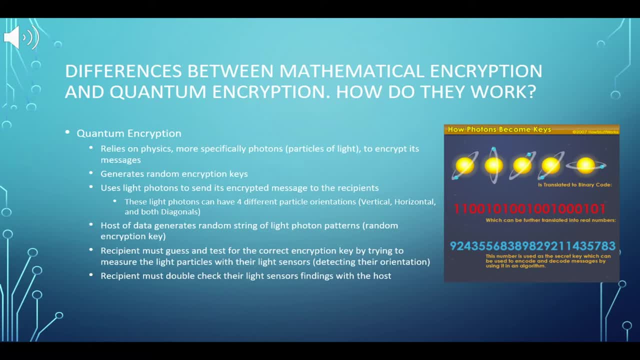 signaling the wrong light orientation to the recipient. This is why the recipient must double-check the photon's orientation with the host to see if they're all right or not. Only if the host knows the true orientation of the light photons the recipient will tell the host what light sensor they use. 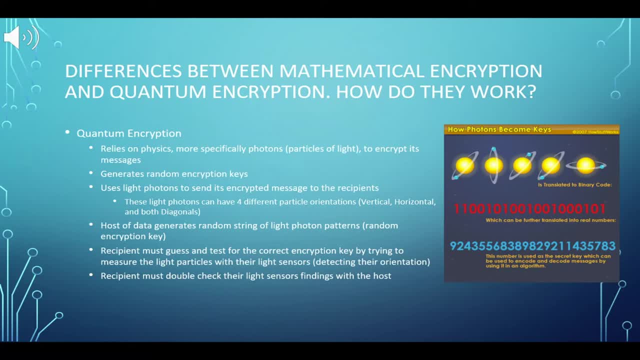 with which light photon and the host will tell them if that was the right sensor to use or not. The host resends the encryption key and the recipient corrects their mistakes and uses different light sensors on the given light photons. Once the recipient gets the correct encryption key, 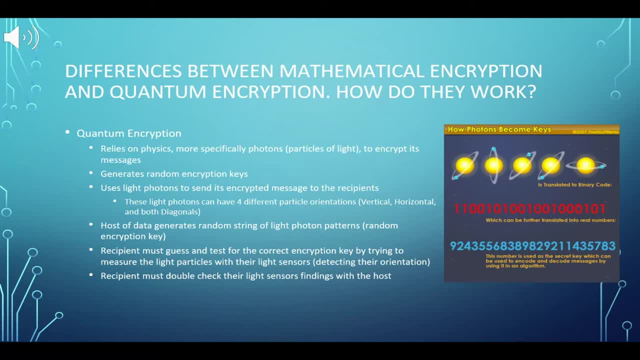 they can use it to decrypt the encrypted message. Another cool thing about this process is the process allows for the host to know when a middleman or a hacker is trying to intercept the encryption process, because it will change the light photon's orientation, thereby letting the host party know. 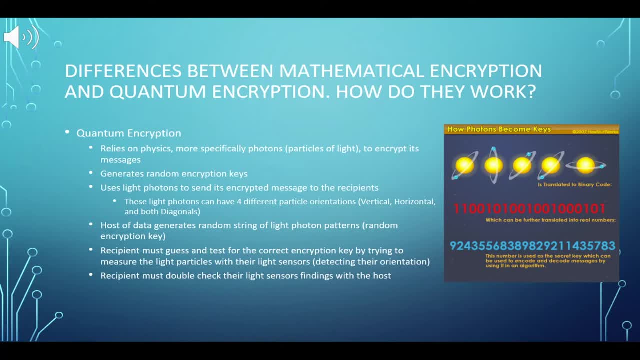 when a hacker is trying to access things that they shouldn't be, Because if a hacker is using the frames that they shouldn't be to try to measure which orientation the light photon is in, if they use the wrong frame, it changes the orientation of the frame. 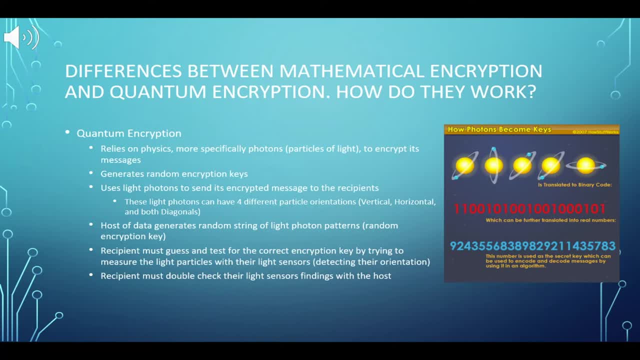 thereby letting the host, once they get the light photon, it lets them know. things have been changed because a middleman is trying to get our information. This is why this technology is more effective and efficient at having a true, secure connection between a host and a recipient. 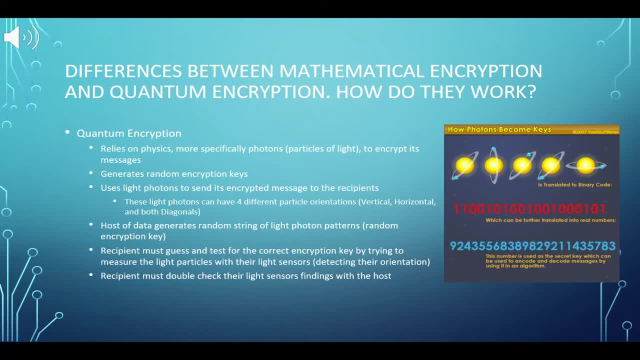 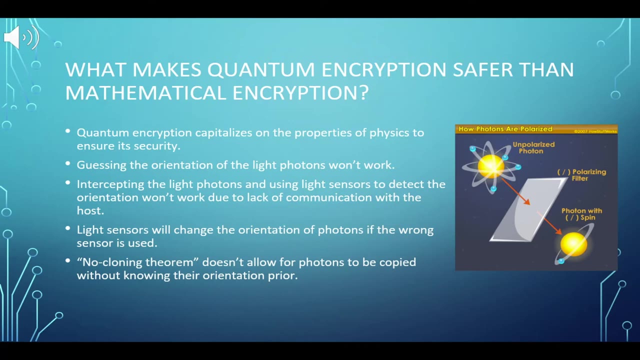 because it truly uses quantum physics instead of mathematical things that computers could eventually break to secure data being transferred between parties. So what makes quantum encryption safer than mathematical encryption? Quantum encryption capitalizes on the properties of physics to ensure its security. Guessing the orientation of the light photons won't work. 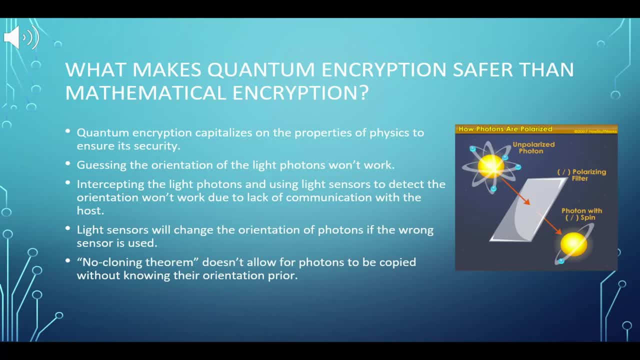 and also intercepting the light photons and using light sensors to detect orientation, won't work due to lack of communication with the host. If you remember the video we played earlier, it demonstrates how you have to communicate with the host after the transmission to basically get the key right. 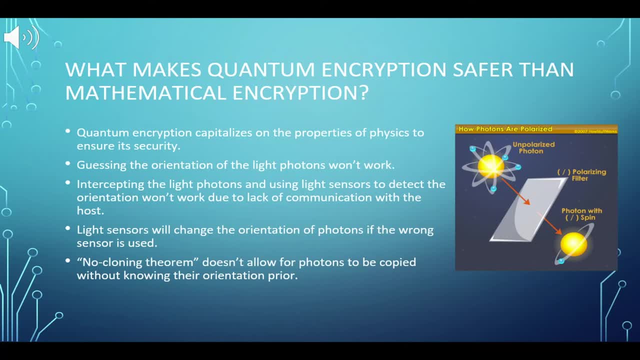 So light sensors will change the orientation of photons if the wrong sensor is used. So this essentially prevents man-in-the-middle attacks, because if someone intercepts a light photon, let's say they use the wrong light sensor, also called filter, let's say they use the wrong filter. 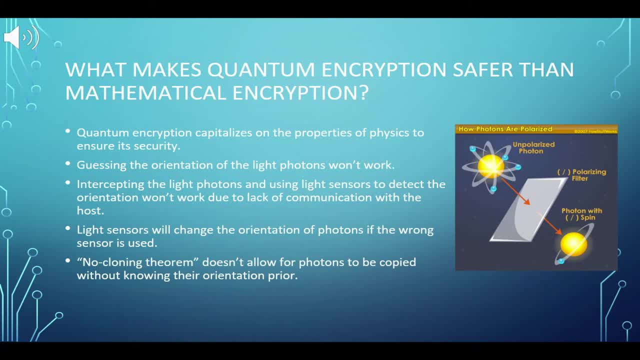 and the orientation of photons change. So when the intended receiver contacts the host and their results don't match up, that photon will be discarded And as well. the no-cloning theorem doesn't allow for photons to be copied without knowing their orientation prior. 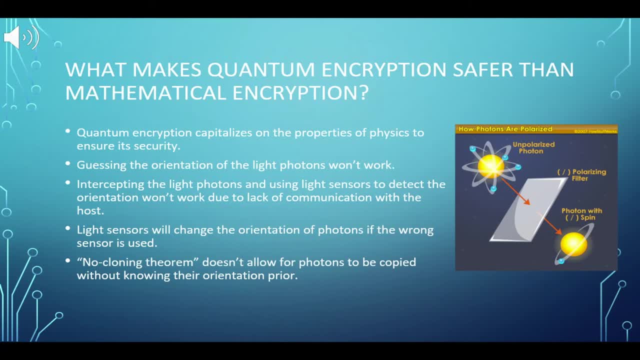 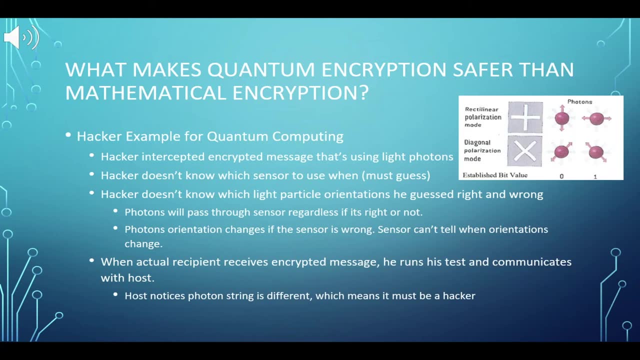 which is very important. What makes quantum encryption safer than mathematical encryption? So below we have an example of a hacker trying to hack into an encrypted message and how quantum computing would come into play as far as him not being able to get it. 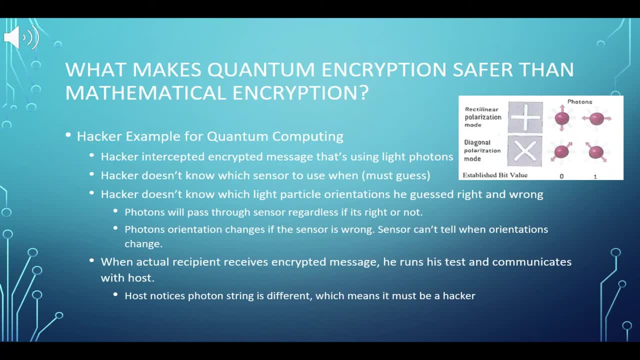 So say, a hacker intercepted an encrypted message using light photons. The hacker doesn't know what sensor to use and the hacker doesn't know what light particle orientations he guessed, right or wrong. So when we send these photons of encrypted data, it's going to go through these different sensors. 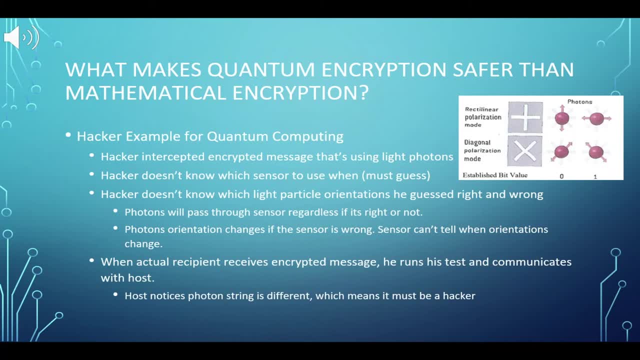 So on this slide there's a small picture in the upper right of the sensors. It either looks like a plus sign or a multiple sign, And when these photons pass through there it will get registered, as you know, rectangular or diagonal. 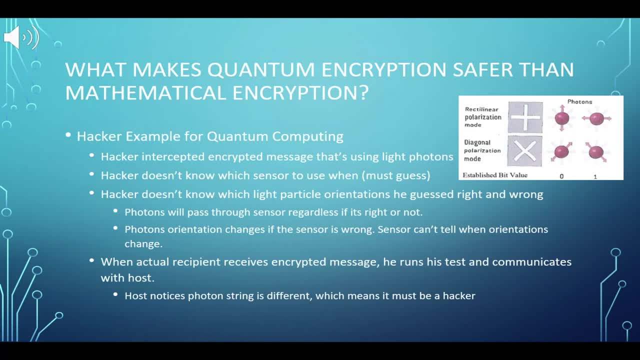 And if it goes in the wrong way, it will be registered a zero or a one. So when you send this message to the recipient, they're going to get it, and the hacker? the only way to know is to put their own filter. 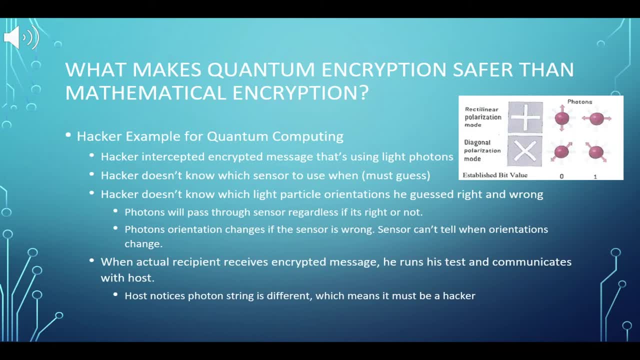 and to see what photon passes through it. So, for example, if he puts a rectangular polarization filter in there and it goes in as diagonal, it's going to get registered as a zero, and vice versa: If it doesn't fit, it will go zero. 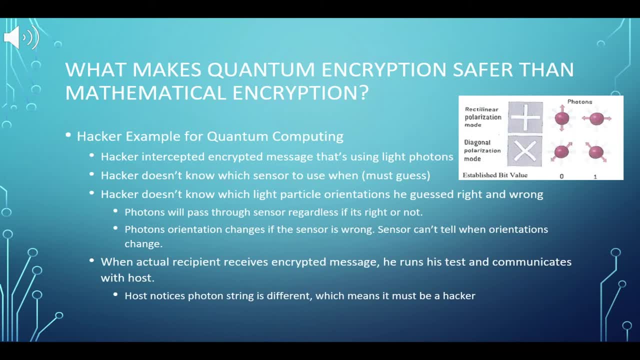 If it fits perfect, it's going to go to a one, So the hacker can throw multiple filters into this and get a string of qubits so that he can decrypt the message. Before he can decrypt the message, though, the host will communicate with the recipient. 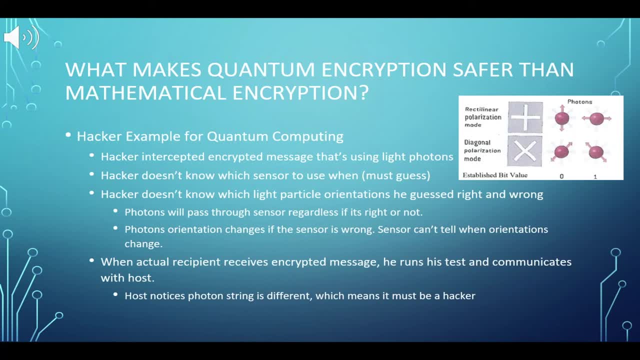 and they will come up with their own sequence as to what was registered and what was not registered. So, off the beginning, the hacker can then know the encrypted data from what the host sent. Now that the host has talked to the recipient, him and the recipient have come together. 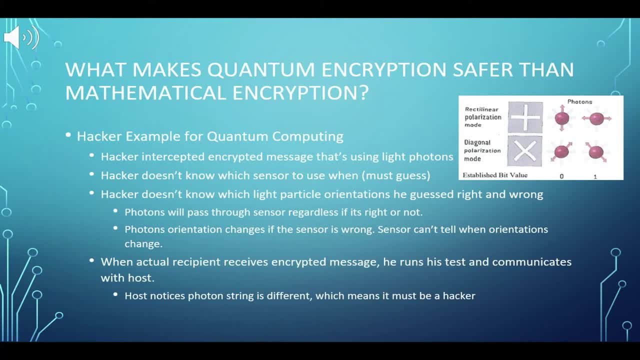 so that the host matches the recipient. Therefore, the hacker no longer matches the host, and only the host and the recipient can communicate through a secure channel where the hacker can really never hack into them. That's the cool thing about quantum encryption: is that it changes based on the recipient's needs. 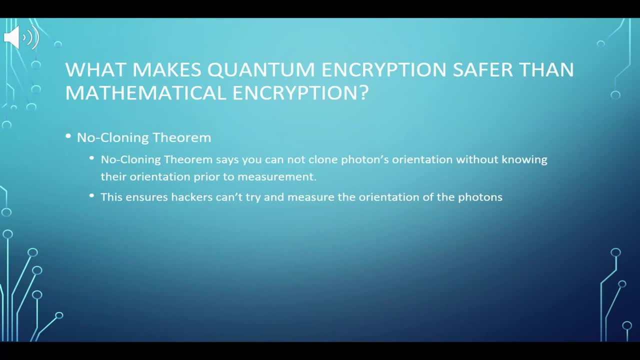 The No-Cloning Theorem. If a hacker were to intercept and replicate a string of photons and send it to the recipient in hopes that the host and the recipient won't notice, this would not be possible due to the No-Cloning Theorem.